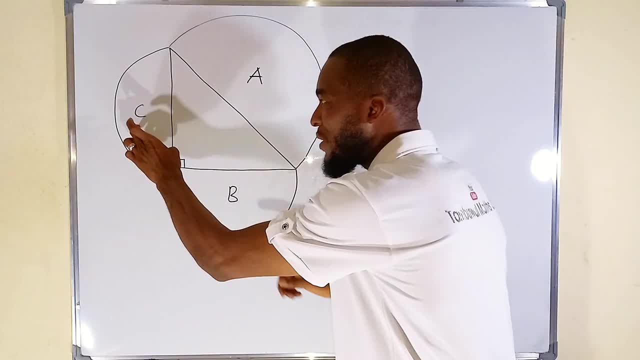 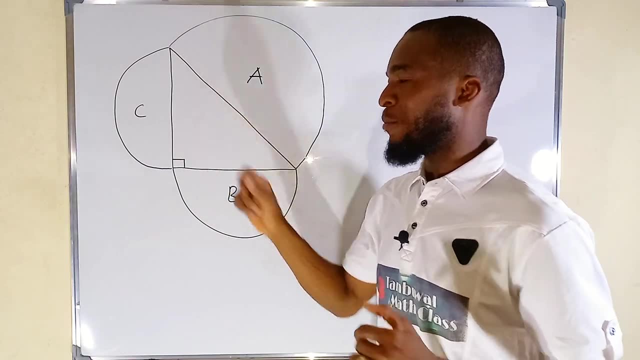 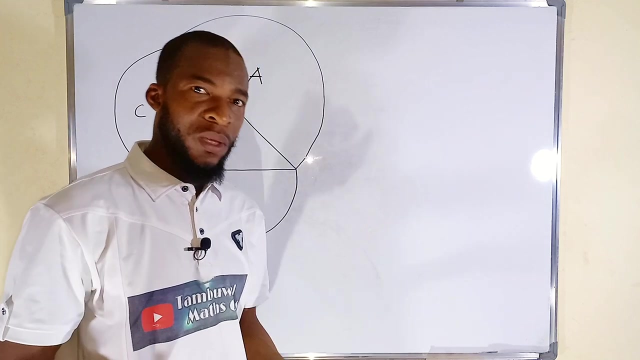 big semicircle, the sum of the area of this C and B, And that's just the question. But if you observe, we have a right angle triangle here. Okay, let's get started. You know, to find the area of a cycle you need the radius, And the area of a cycle divided by two will. 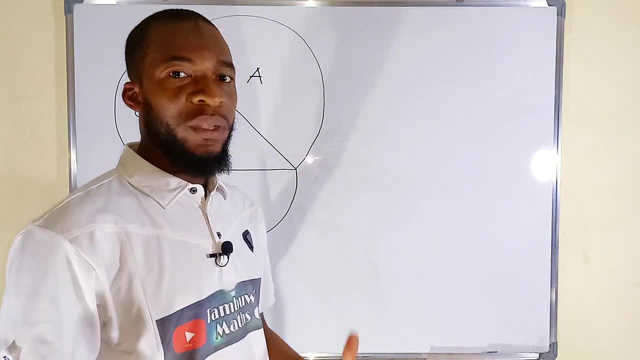 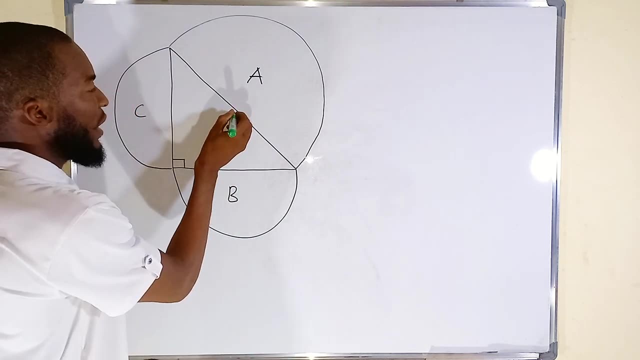 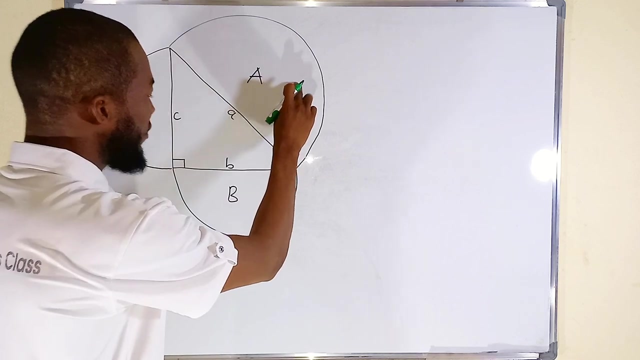 always give us the area of semicircle, because semicircle is half of a cycle. So since we don't know the length of these respective sides, let's call this one A, let's call this bigger semicircle, BC respectively. So let us first of all find the area of this big. 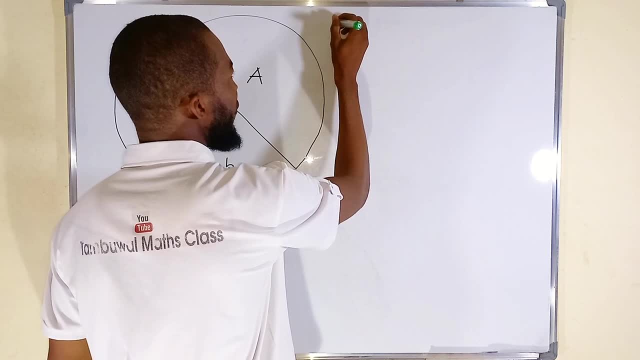 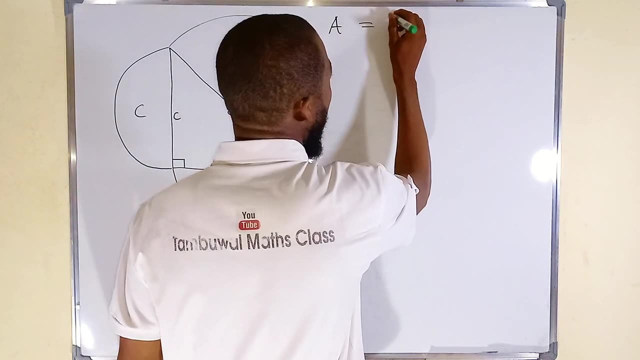 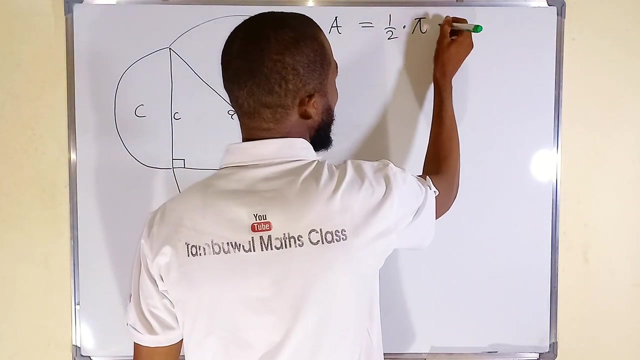 semicircle. It is going to be for, let me say for A. it stands for the area of this. It is equal to half, because we have to divide the area of a cycle by two. therefore, half multiplied by pi, then multiplied by r squared. But what is our r? 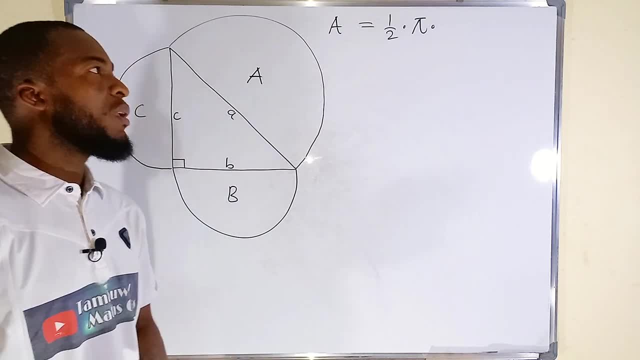 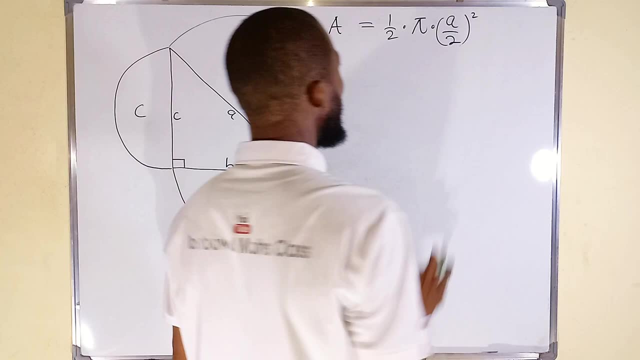 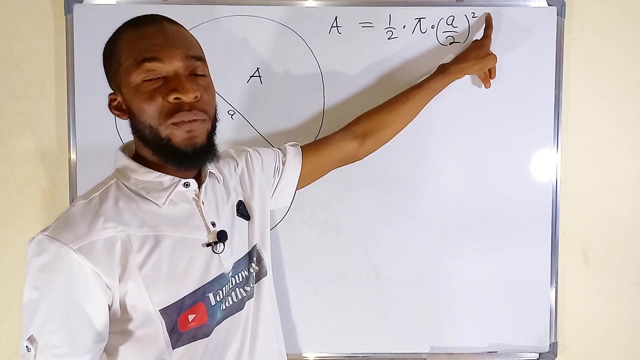 r will be A divided by two, because diameter divided by two is equal to the radius. So we have A divided by two, whole squared. So this is what we need to simplify to obtain this area. You know, A to the power of two is A squared. two to the power of two is four. So we have: 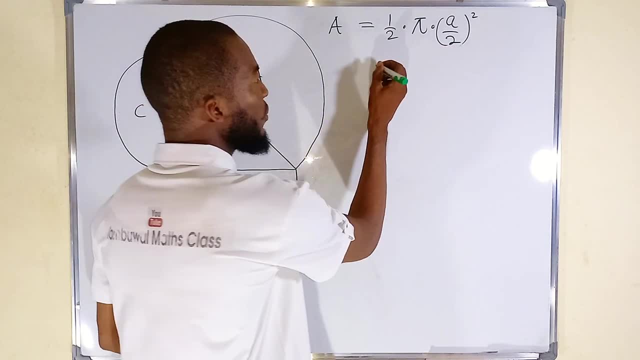 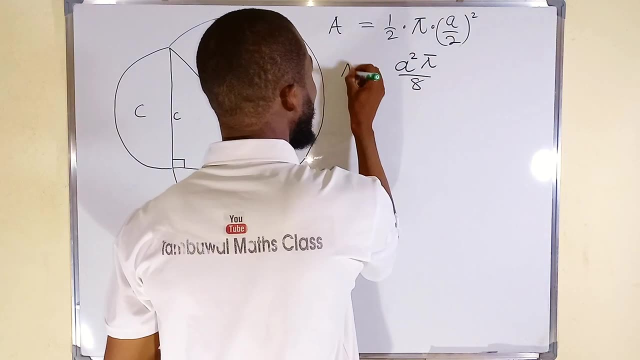 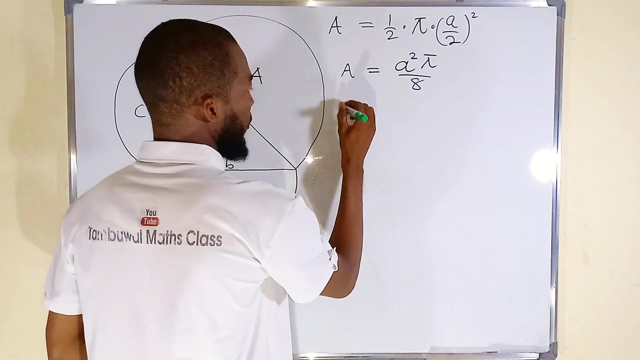 two here, multiplied by this four, it is going to give us eight. So altogether we have A squared pi over eight. So this is the area of this big semicircle. So we are going to do the same thing for all. For the b it will be half pi. what is the diameter? 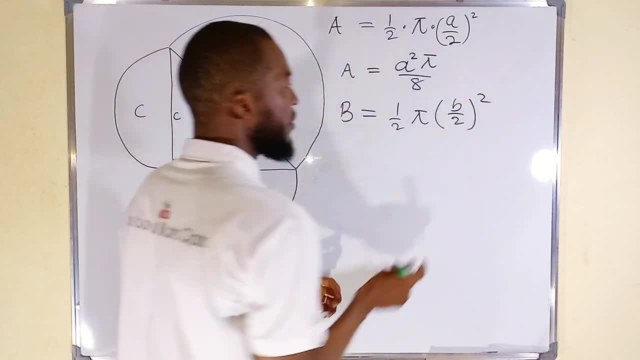 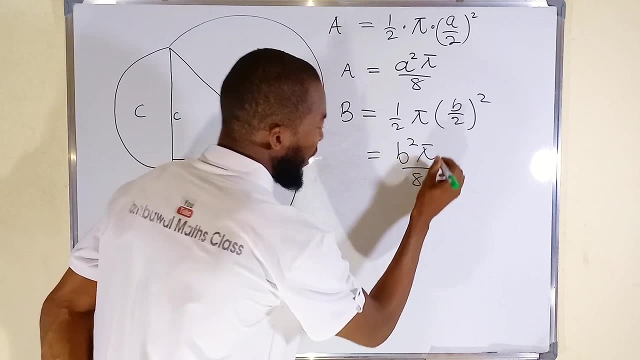 B divided by two squared. To simplify this, you are going to obtain b squared pi over eight. and for the last one, this question is very simple. For the c part, this is equal to well. our rib did not go away. This we. 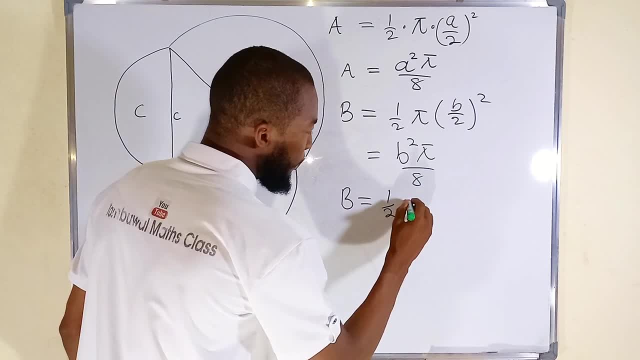 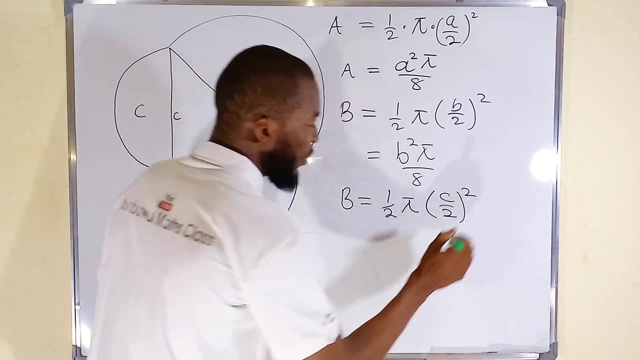 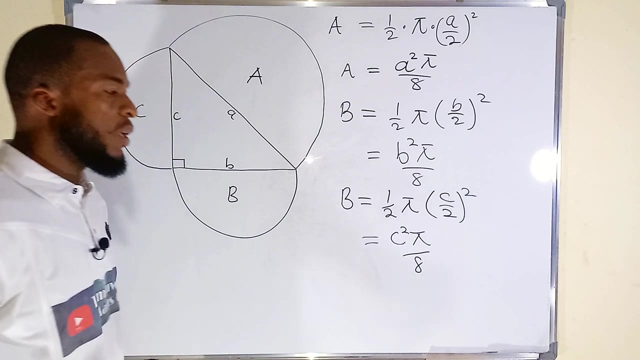 call the angle square, So you can look at it from this side and you will have the six punctuation values: two half pi, then the diameter is C divided by 2. we get the radius R squared. multiply everything, you have C squared, pi over 8. so these are the respective.